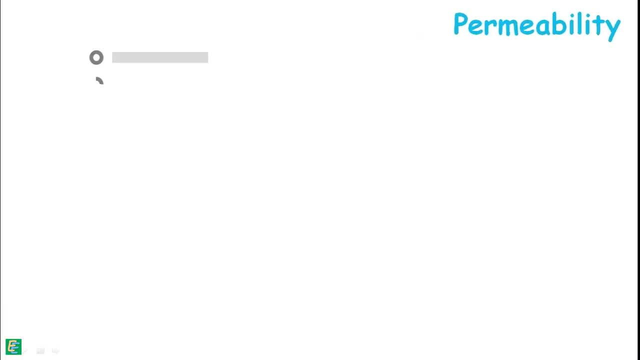 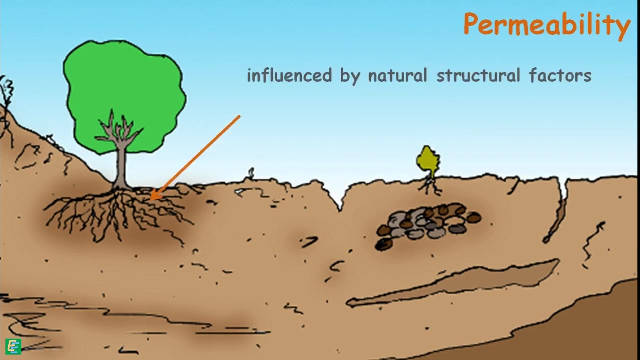 property. There are numerous methods through which we can measure the permeability of a soil in the field or of a representative sample in the soil. We have already discussed laboratory methods. Permeability of the soil in its natural deposits is highly influenced by its natural structural factors, such as non-homogeneity and stratification. 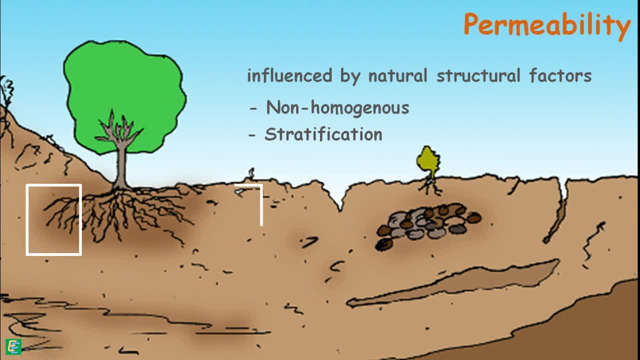 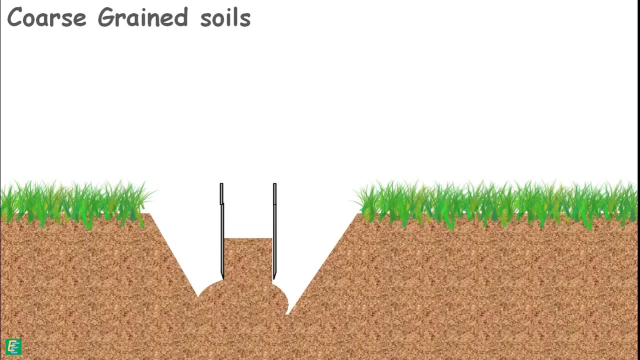 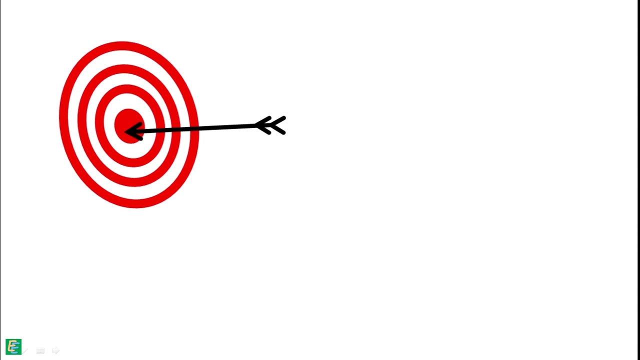 So it is not possible to take out a soil sample which may represent the true in-situ structure of the soil to be used in the laboratory- Most grain soils in which permeability values are very significant- it is very difficult to obtain undisturbed sample. So to deal with such problems and to obtain a near accurate 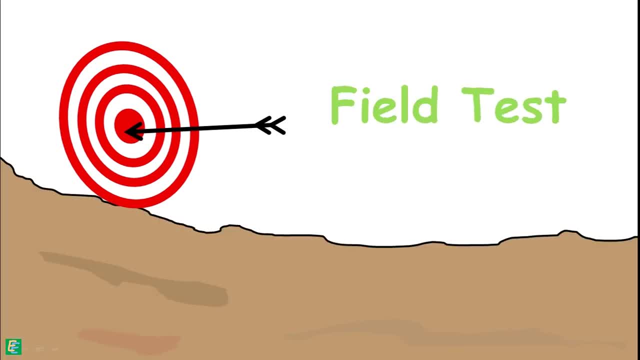 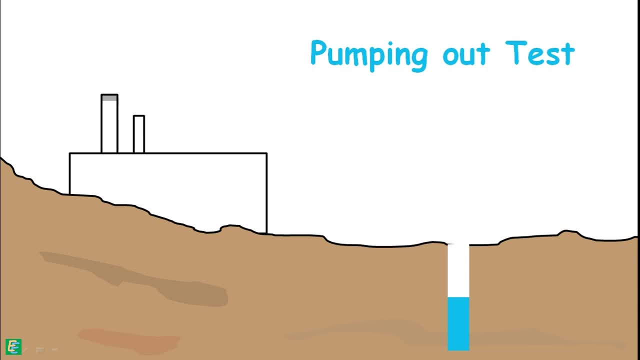 value of permeability. we perform field tests on the soil mass. Usually, pumping out test is conducted for the purpose. We perform these tests for large engineering projects because these tests are very expensive. The soils in the ground are the reservoir of the groundwater. Their voids work as a storage. 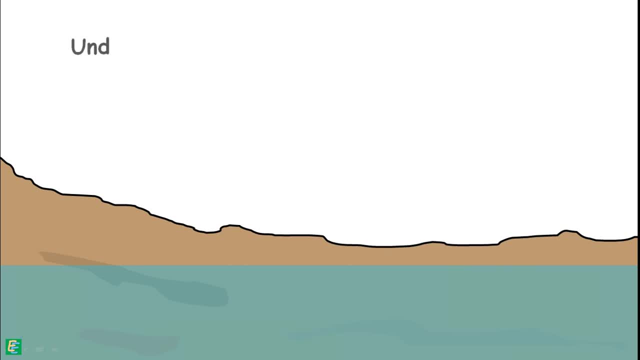 and passage for the water. Such an underground layer of permeable rock or unconsolidated material, such as gravel, sand or silt, is called an aquifer. It is a body of saturated rock through which water can easily move. The groundwater from the aquifer can be easily pumped out. 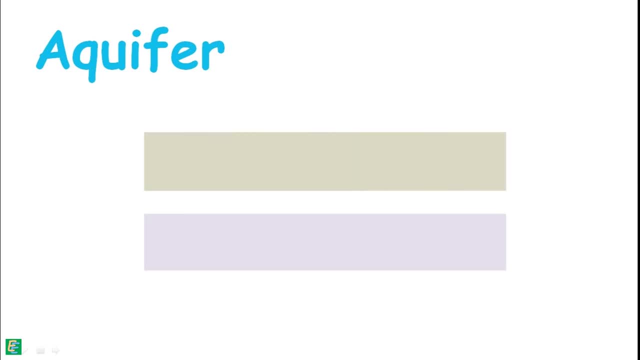 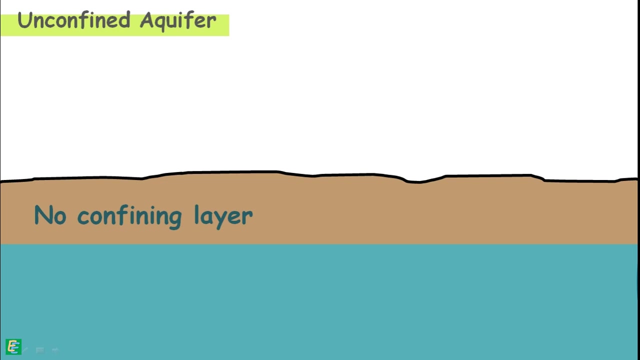 We usually encounter two kinds of aquifers. One is unconfined aquifer and another one is confined aquifer. Unconfined aquifers simply means an aquifer that does not have a confining layer between it and the ground surface. Water can flow directly between the surface and 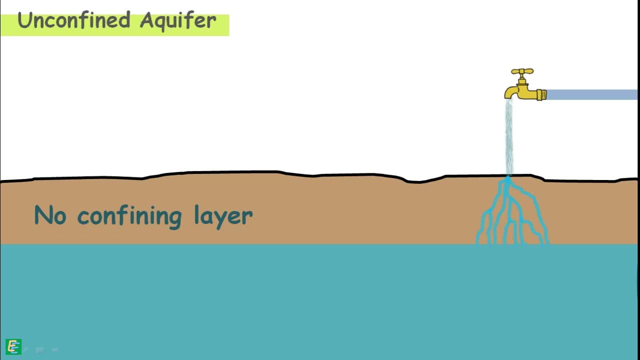 the saturated zone of aquifer. An impervious layer may present under the aquifer but not above it. Unconfined aquifer remains at the atmospheric pressure. These aquifers are sometimes also called water table aquifers because their upper boundary is the water table. But sometimes 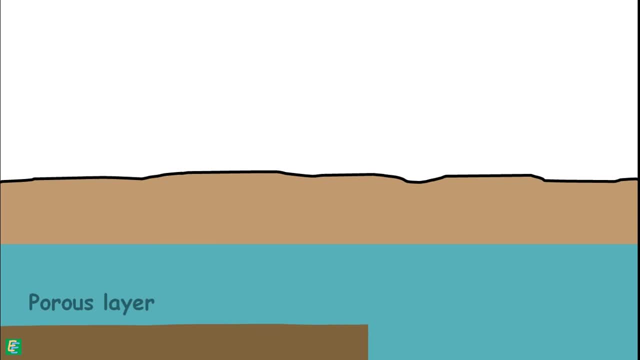 this porous water holding layer is confined or sandwiched between two impervious layers of soil, and the aquifer is bounded at the top and the bottom by relatively impermeable strip. In such aquifers, water cannot enter or leave by a vertical flow because of these impermeable 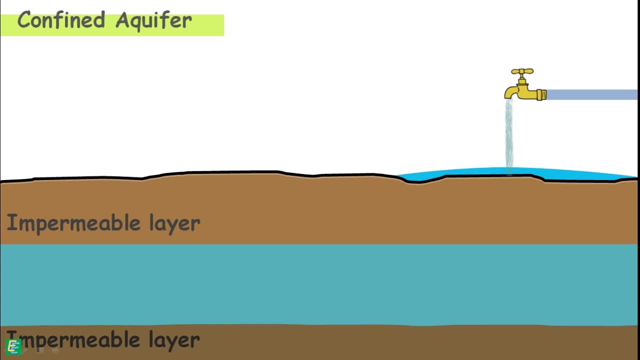 soil layers. These impervious layers of soil are called aquicludes, and these are often made up of clay soils. Under such conditions, water may also be present in the pressurized state. When a well is drilled into such aquifer, the internal pressure pushes the water up. 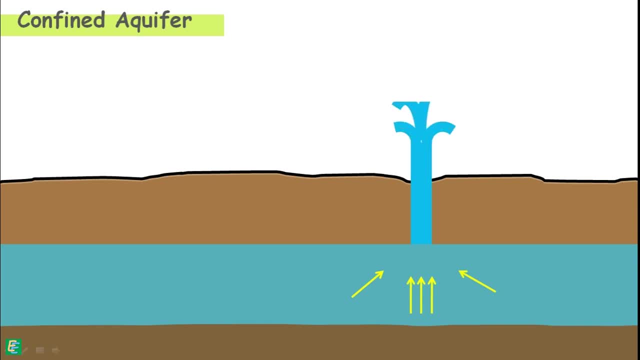 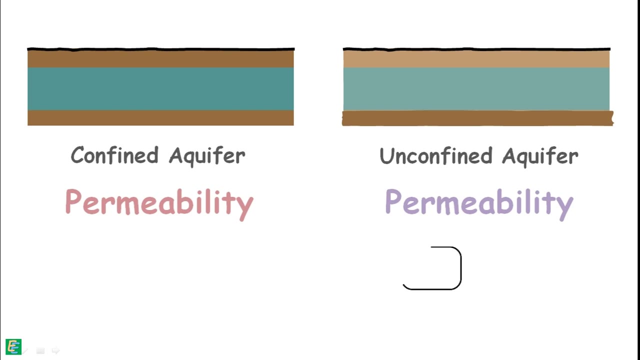 and in some cases water even comes up to the surface completely out of the well. This type of well is called artesian aquifer. For both confined and unconfined aquifers, permeability calculations will be slightly different. We have already discussed the permeability of unconfined aquifer. Now we will discuss 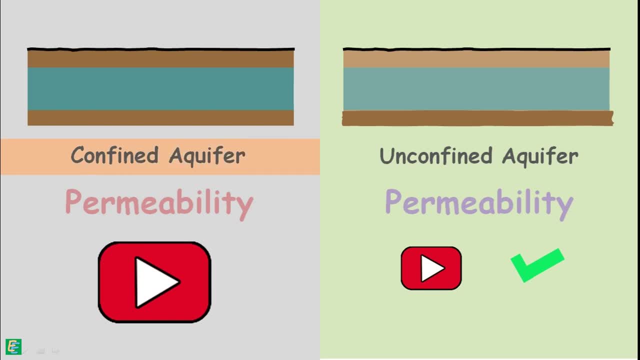 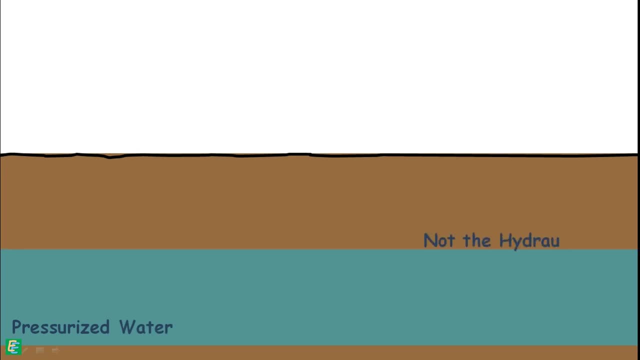 the permeability of confined aquifer. In confined aquifers water remains in pressurized state. The thermal level of the aquifer is not its hydraulic head, Because we know total head or energy of the water is the height of the water column plus its pressure head plus. 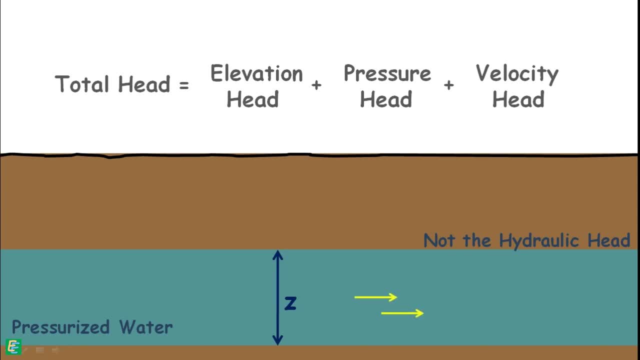 velocity head. Velocity of water inside the soil being very small, velocity head is neglected And energy of the water only remains its height and pressure. So the actual energy of the water can be measured by inserting a piezometer. Let me give you an example of the energy level of the water column When the water is connected. 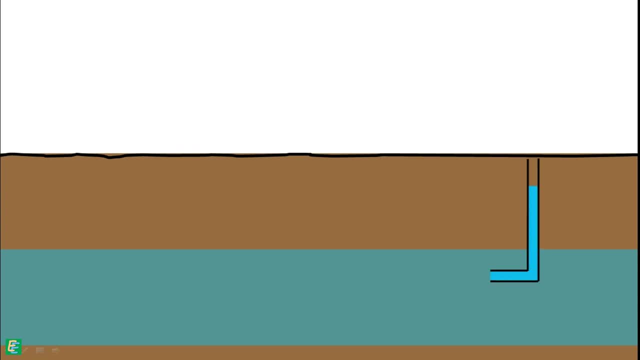 to the pressure level of the aquifer. it uses the pressure value to evaluate the water as the boost. The flow rate is the amount of pressure of the water by the amount of water Now, for example, at any point in the aquifer and reading the piezometric head, or by making an 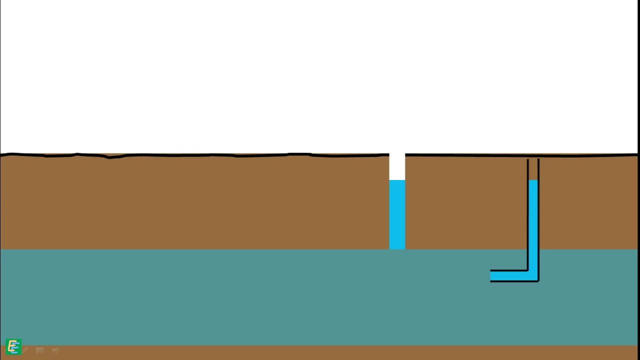 observation well into the aquifer and measuring the water level in it. We may draw a piezometric surface or energy surface above the aquifer, which may indicate the hydraulic head of the aquifer. We can notice this is above the actual water level. In order to measure the permeability of such aquifers, we 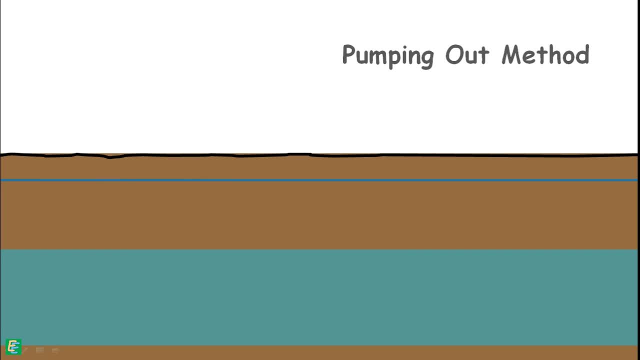 employ pumping out method. Pumping out method involves making a well into the ground that reaches the aquifer and penetrates it throughout its whole thickness. It is important that well penetrates the entire thickness of the aquifer. It is called test well. Water is pumped out through this well and as a 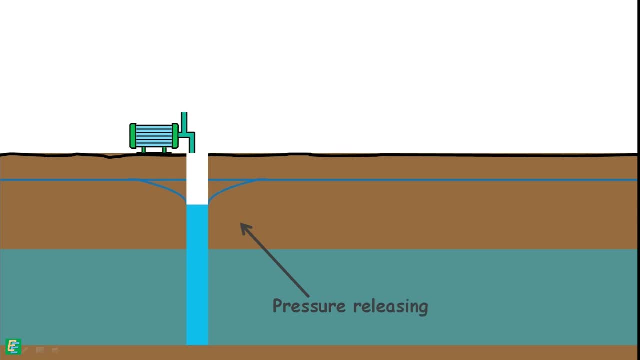 result: pressure of water starts releasing and piezometric level starts decreasing. The piezometric surface of water, which may be horizontal initially, is then acquires this kind of shape that is called cone of depression. We can observe this by making two observation wells at some distance from the test. well, We can measure the difference of 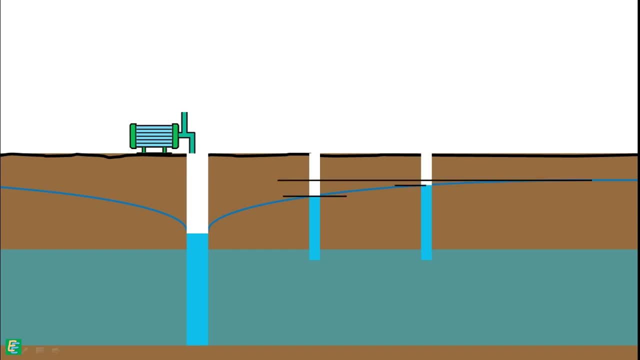 water levels in them before and after the water has been pumped out of the well. When the water is pumped out, a hydraulic gradient is formed inside the soil mass because of the piezometric profile generated. The height of the piezometric level at any point is the hydrolic energy or. 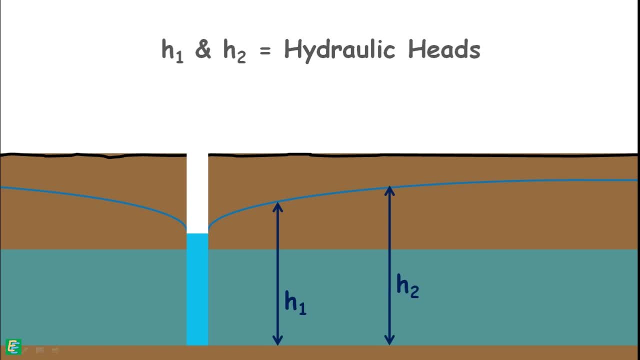 hydraulic head of the water. at that point We know water flows from high hydraulic head to low hydraulic head. The water level in the well may be higher than its surrounding, but it has lower head than its surrounding. So water will flow from all directions: of high head into the well of low head. If we imagine it in 3D, see the flow is radially inward from all directions. Hence, when we pump out the water from the well, the water in the aquifers moves towards the well and starts refilling it, But still we continue the pumping of water till the steady state of flow is reached. 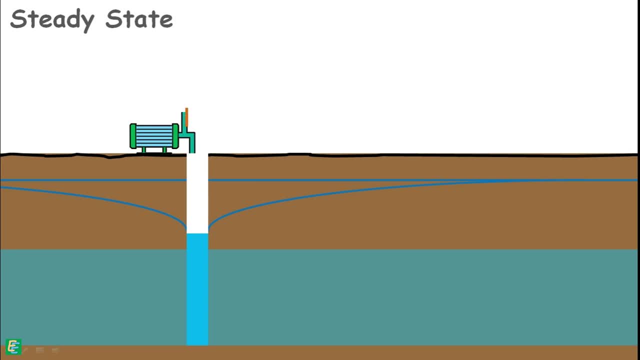 The steady state of flow is reached when the amount of water pumping out from the well becomes equal to the amount of water refilling the well. So rate of water radially crossing in this cylindrical surface is equal to the rate of water entering into the well, and that is also equal to the rate of inflow water from this. 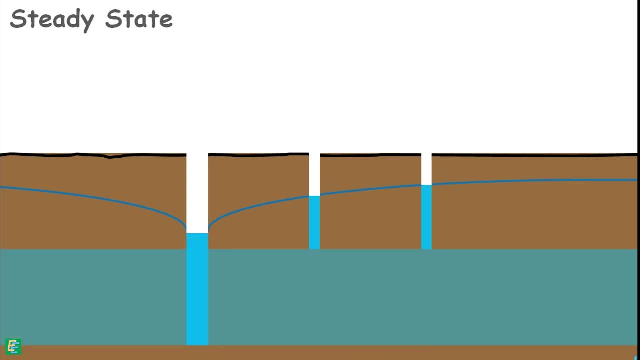 cylindrical surface. At this state water level in the well will not change. In such a state the drawdown curve becomes constant and the water level in the observation wells also increases. So let at this steady state the height of the piezometric level in the first observation. 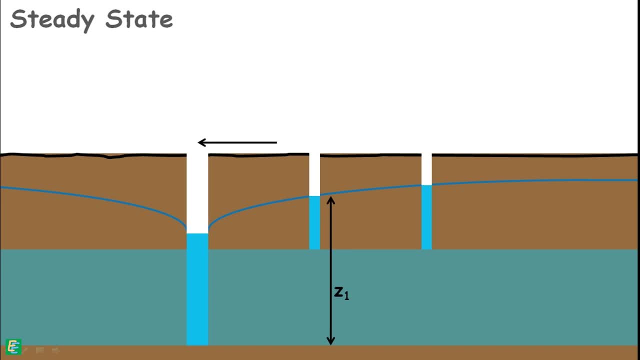 well is Z1, and it is at a distance of R1 from the centre of the test. well, Similarly, the height of the piezometric level in the second observation: well, is Z2, and it is at a distance of R2.. Also say the thickness of this confined aquifer is capital B. 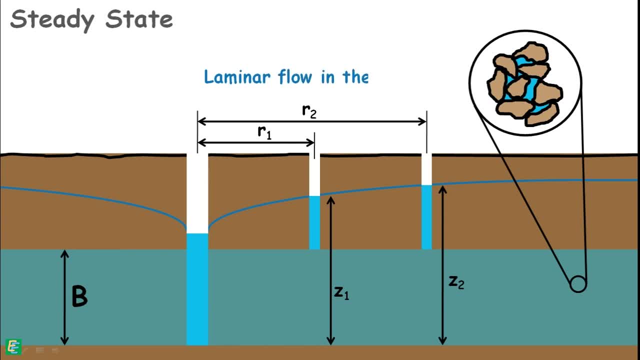 We assume that the flow of the well is constant, But the flow of water in the soil voids is laminar, So we can apply Darcy's law for this situation. According to the Darcy's law, discharge rate from the well Q is equal to the permeability. 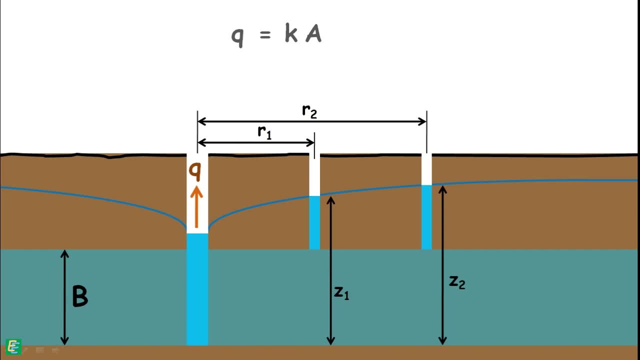 of the soil, multiplied by the area through which the water is percolating, multiplied by the hydraulic gradient which is causing the flow, We can see the hydraulic gradient has a curved profile. It is not constant. Let's assume that at some distance R from the centre of the well. 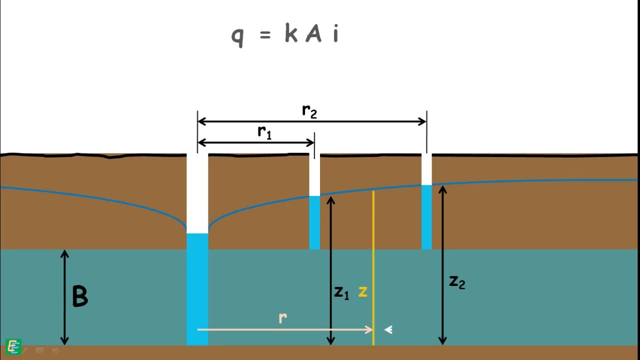 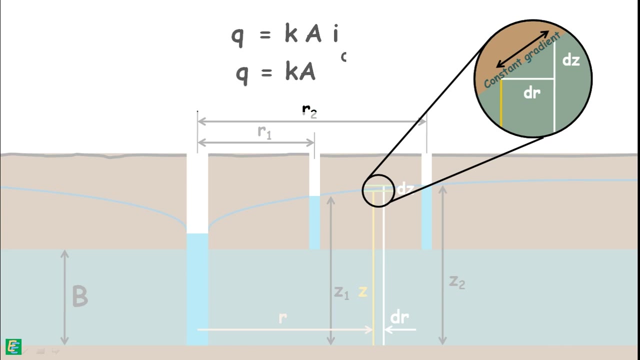 Pcie th level is Z And atsc distance DRw. the height of the piezometric level increases to dz height. For such a short distance we can consider the hydraulic gradient as constant and that will be equal to change in piezometric level divided by the distance over which the change. 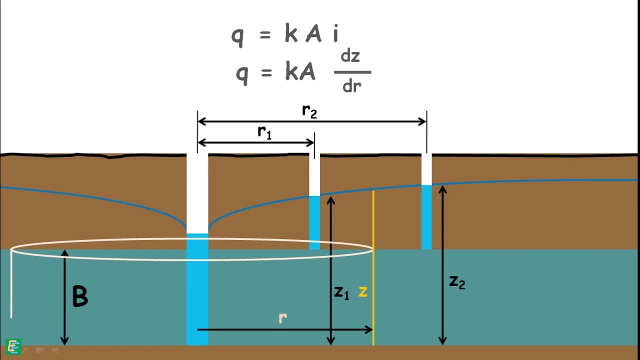 occurred. A화를 the distance across which the water is percolating. anda target Hong water is percolating by this hydraulic gradient. is this cylindrical surface of radius R and height capital B, which is the thickness of the aquifer. So area of this cylindrical surface is 2 pi R B. 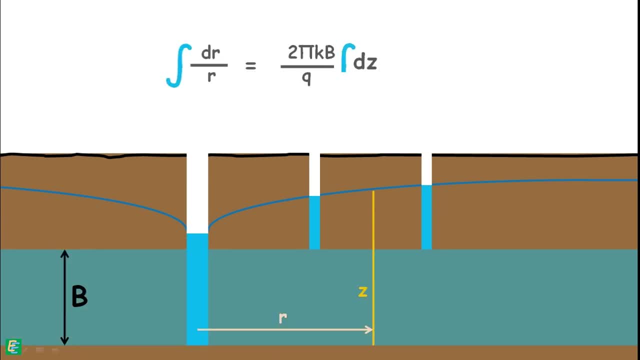 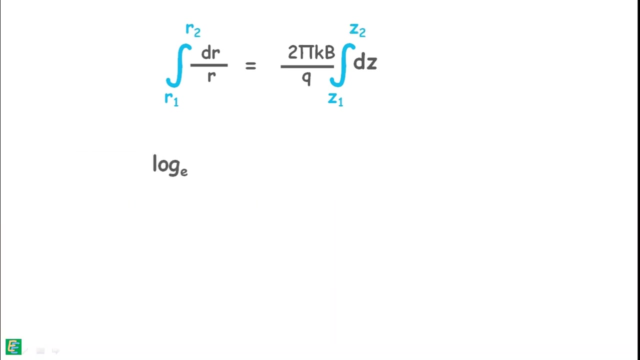 Rearrange it like this And we can integrate it from our observation of water level in the observation well, which was at R1 distance from the test well, was Z1, and level in the well which was at R2 distance was Z2.. After integrating and applying limits, we can find the equation of permeability of the soil. 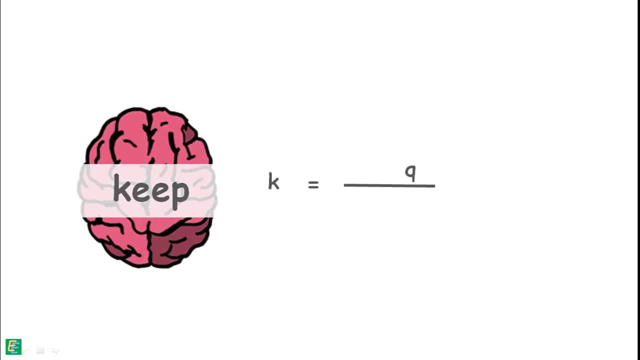 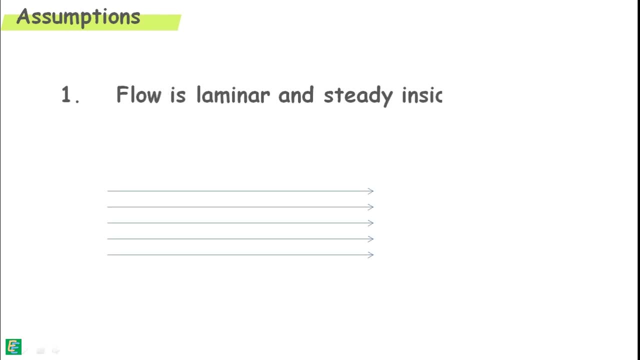 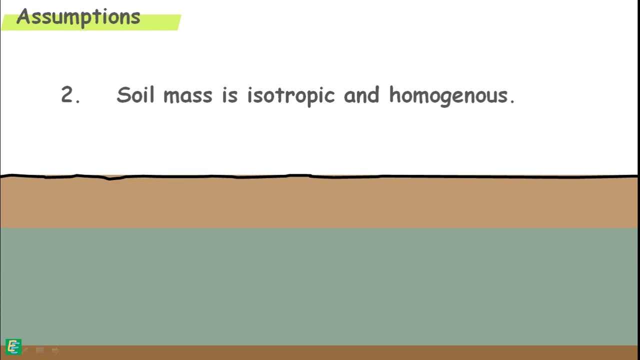 We should keep in mind that, in obtaining this value of permeability of the soil, we have assumed certain things. First, we assumed that the flow is laminar and steady inside the soil. Second, we assumed that the soil mass is isotropic and homogeneous.